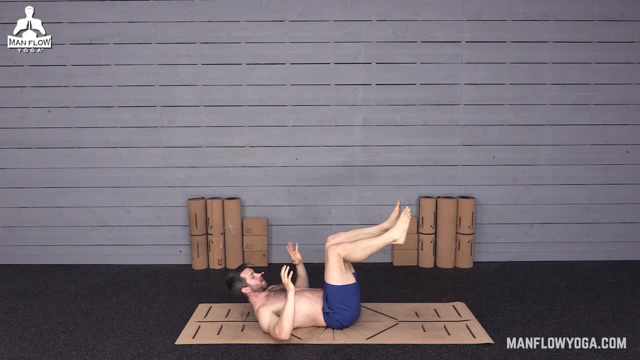 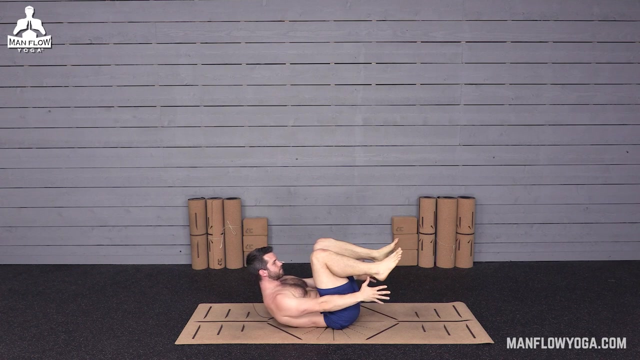 We're gonna get started here on the ground, working your core. So this is really important for weight loss: getting your core engaged. getting your core engaged, getting your core engaged, Getting that sensation of your muscles working, Building muscle, is what's going to help with weight loss. The more muscle you have, the more fat you burn, even while you're not working out. 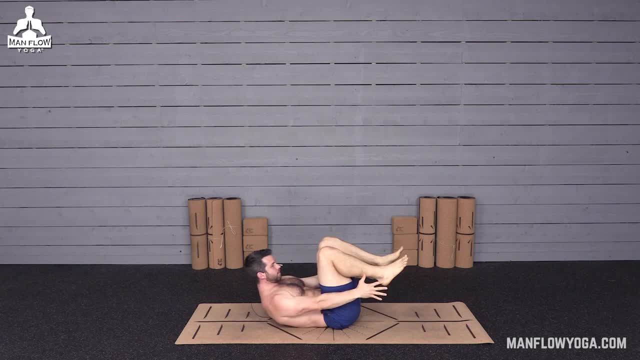 So focus on the muscle, focus on getting the right technique, and the weight loss is going to follow. Alright here. plant your feet in front of your hips, push down through your feet, lift your hips into a bridge, and you can also bring your arms straight up to make this a little more challenging. 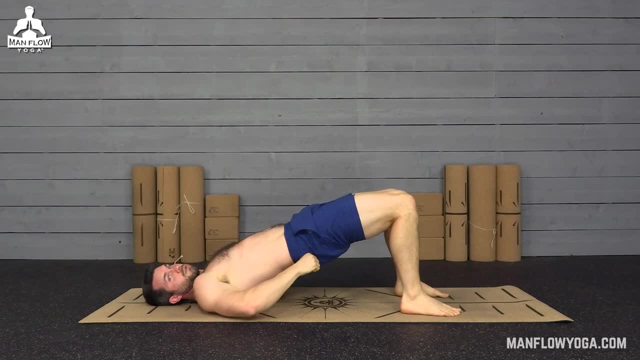 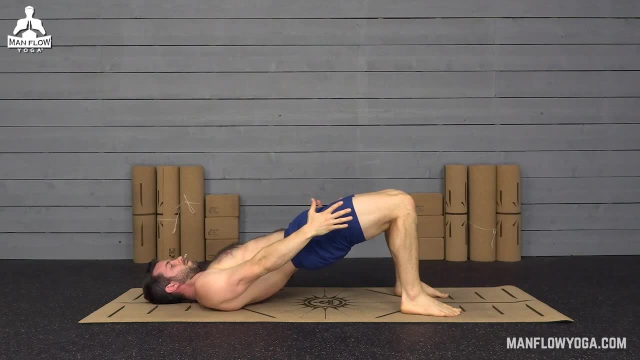 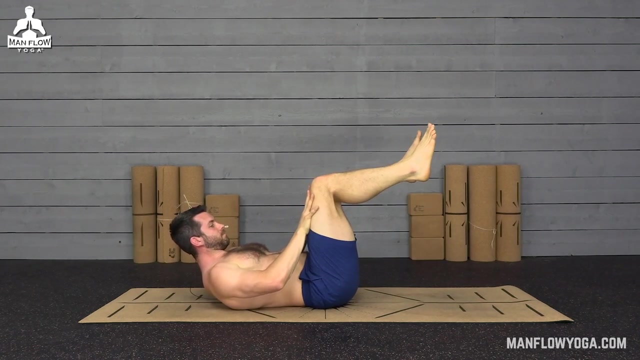 10 more seconds here. squeeze as much as you can, push down through your feet, squeeze your thighs and then release down. all right, bring your knees back over your hips. now we're gonna press your hands into your thighs. push your thighs back into your hands and resist with both. so really push your hands hard. 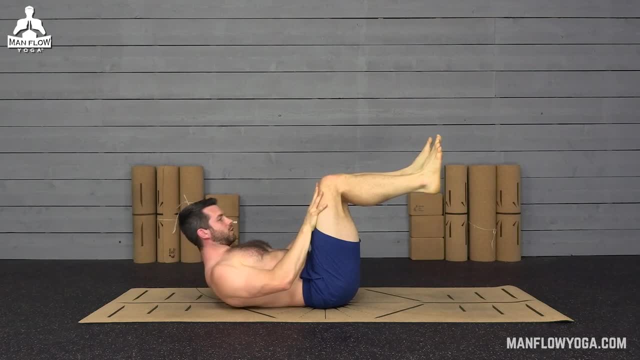 into your thighs. press your thighs back into your hands, lift your shoulders off the ground. and just 30 seconds here, but push as hard as you can remember. we want to make the muscles burn. that's gonna help you with losing weight. it's not gonna be breathing fast or moving quickly. it's gonna be building muscle. 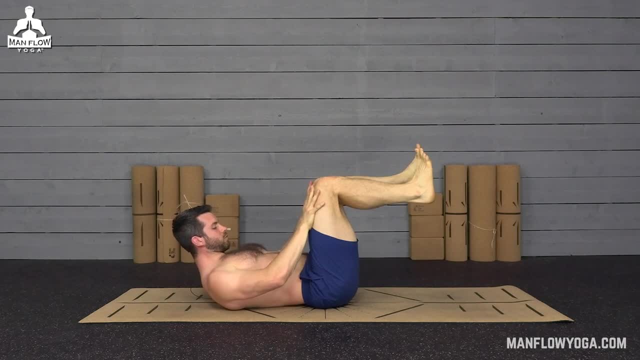 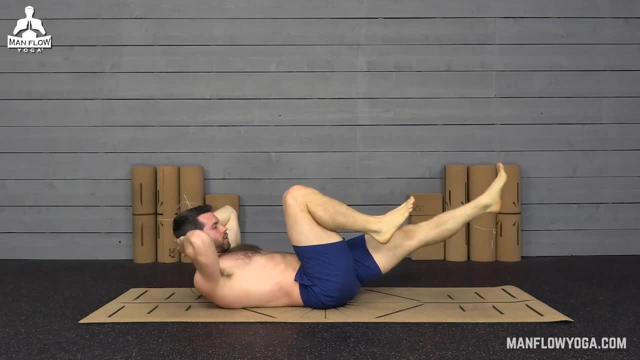 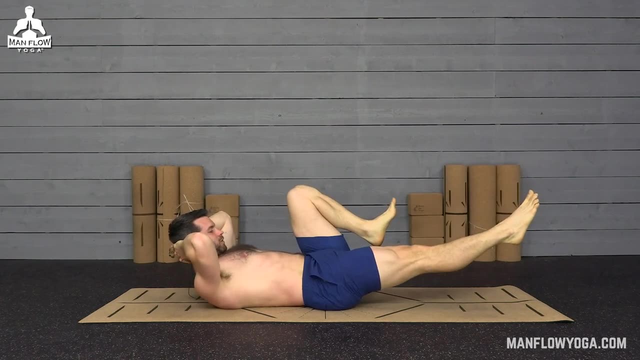 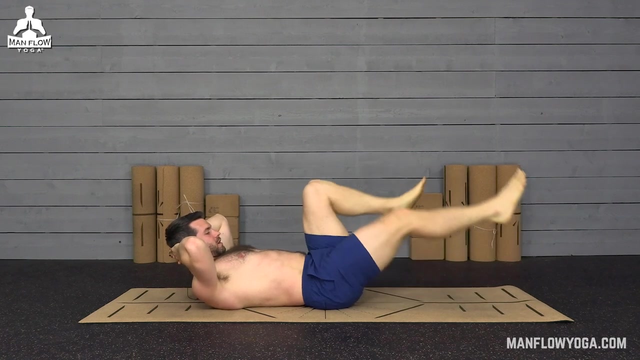 shoulders a little higher and then switch sides. one breath here, switch, switch again and then go back and forth like this just for 30 more seconds. to make this more challenging, bring your elbow to the opposite knee as you're switching sides. try to keep your breathing consistent. 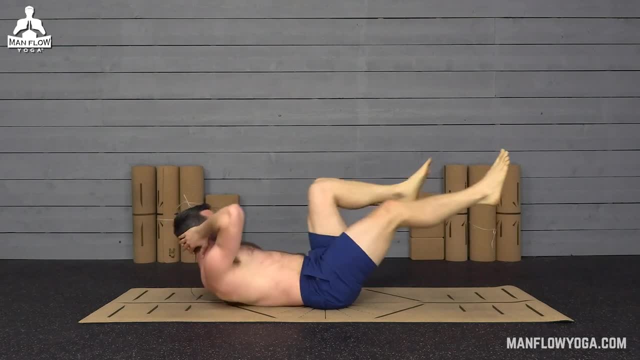 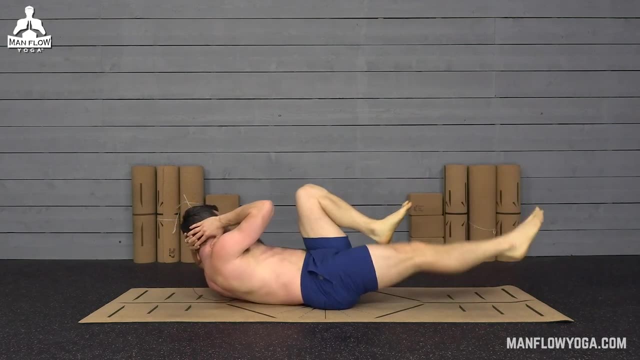 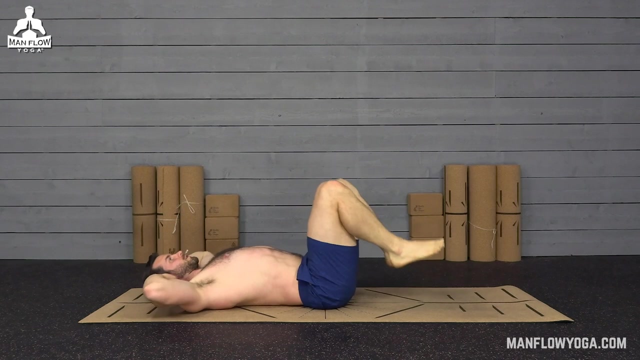 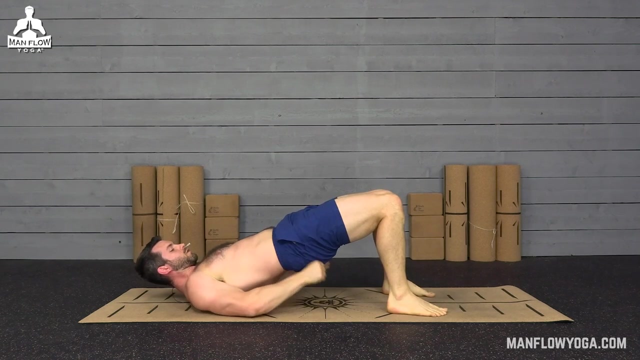 get your shoulders higher to make this more challenging. ten more seconds. knees back over your hips and release down. all right, I'm here, you're gonna push down through your feet. come back up into a bridge. make sure that your thighs are squeezing toward one another. really squeeze your butt here, your butt also. 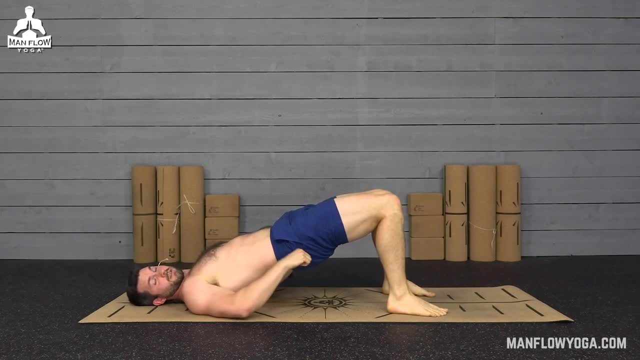 really important for weight loss: getting those muscles back into your thighs and getting those muscles working so that the rest of your body functions properly and we don't get injured and have to skip. workouts from here you're gonna bring without moving your hips. bring your left leg straight out in front of 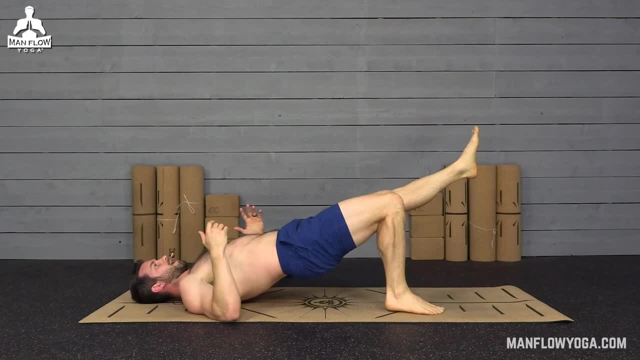 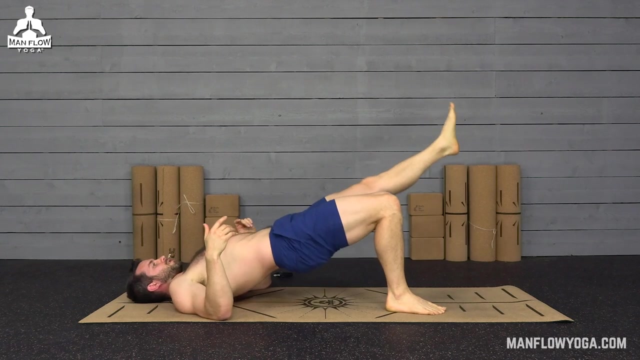 you hover it about a foot off the ground and now we're gonna add in some pulses. so inhale to bring your hips slightly down. exhale, drive up, do ten of those. so you're trying to drive your hips up as high as you can as you exhale, inhale. 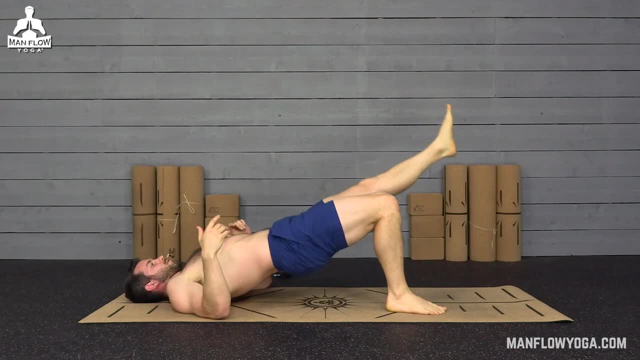 in the inhale. same thing, היאing to release a little bit about five more. make sure you're pushing down through your whole foot using your hips, not trying to rely on your shoulders- and then hold it at the top for ten seconds as hard as you can really squeeze. five seconds, one breath, and then plant your. 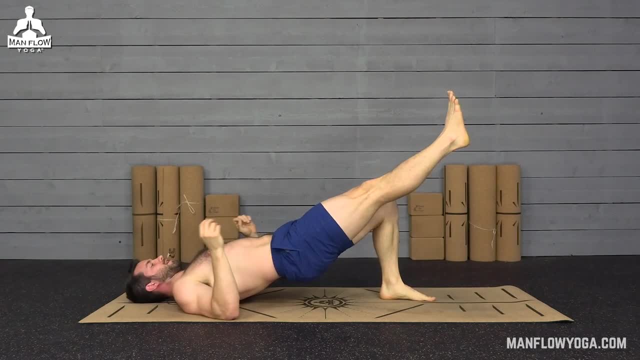 left foot, bring your right foot out and we're going to go straight to those pulses again. so ten pulses coming down, exhaling, press up and going up. thank you up. make sure you're pushing with your hips here, not pressing up with your back, but squeezing. 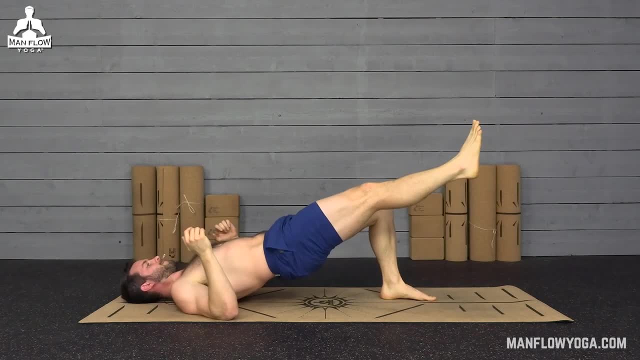 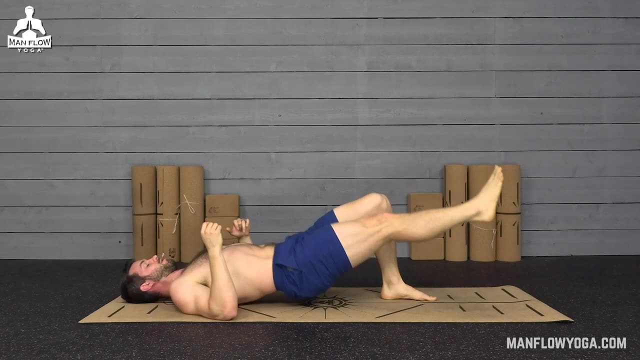 your core and your hips, So there's minimal pressure on the back here. This is a really good exercise for your glutes. It's going to help with actually toning your glutes, building strength there. It's also good for your breathing. 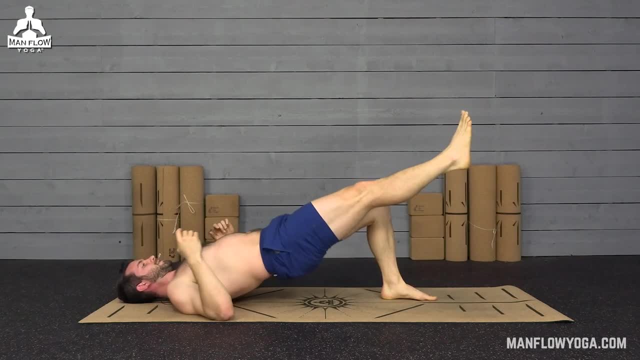 good for your core, your knees, your back. This is just a really good exercise for a lot of different things. All right, coming up to 10 here. you're going to hold it for 10 seconds. Hold that leg out. 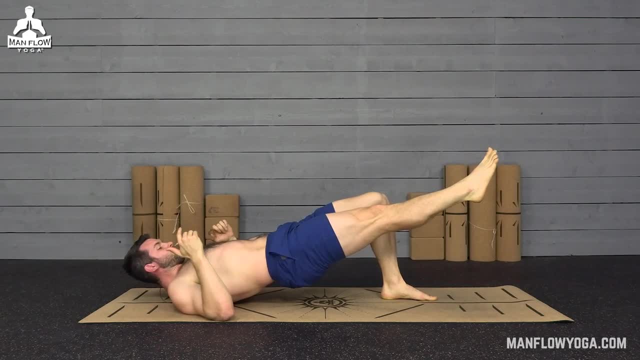 Make sure it's not too high. Just keep it a foot or so off the ground. Try to control that breathing Guys, stick with me here. This is going to be a fun workout. We've got a lot of really cool exercises. 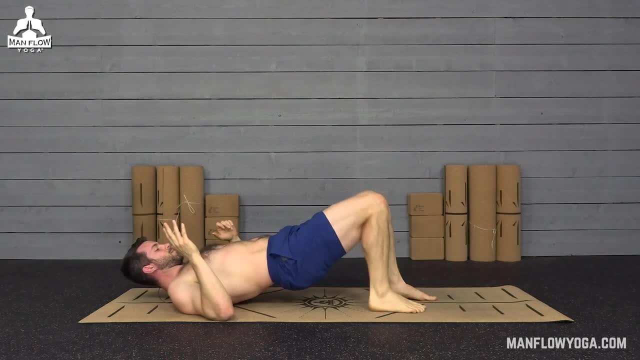 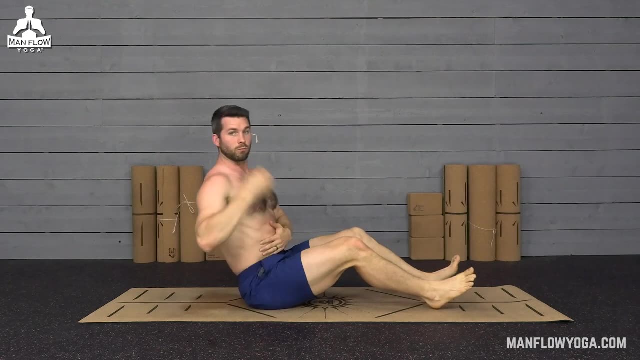 so stick around to the end- It's not that long- And then plant your foot and release. All right from here we're going to move up into a seated position. This is called a boat pose. It's really good for your core and building strength. 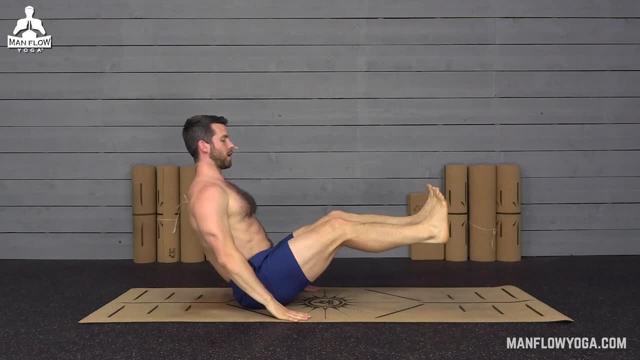 in your core is really important for weight loss here. So we're going to bring your shins parallel to the ground. Lift your chest up If you need to. you can use your hands on either side of your hips to help support. Make sure that your chest is open. 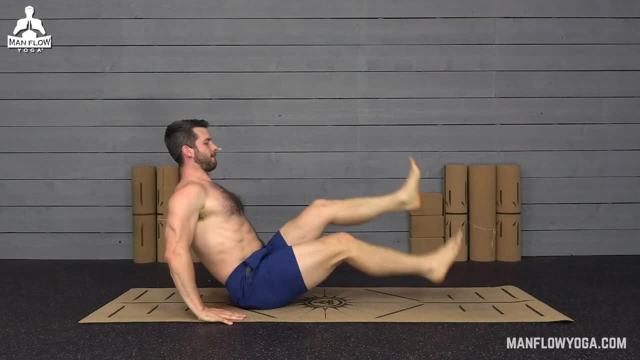 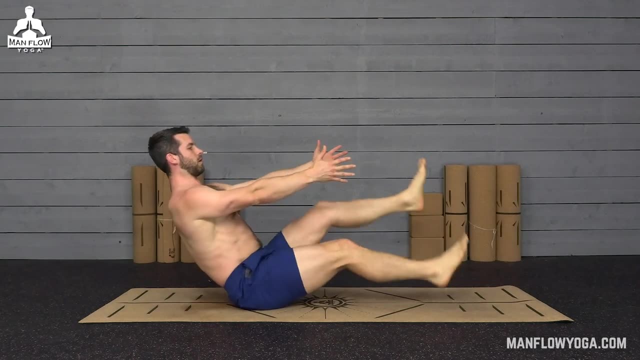 And then from here you're just going to move your legs up and down. keeping yourself in this upright position, You can use your hands to help support yourself. If you want to make it a little harder, bring your arms out in front of you. 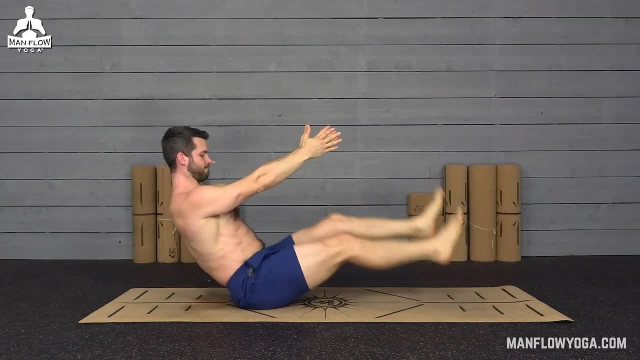 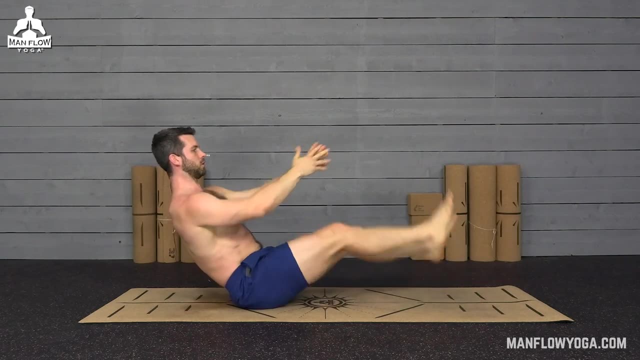 And we're here for a total of 30 seconds, so probably got about 15 more seconds to go here. Keep your chest upright, Try to keep your breathing in control. You're going to feel your hips working, feel your abs working. 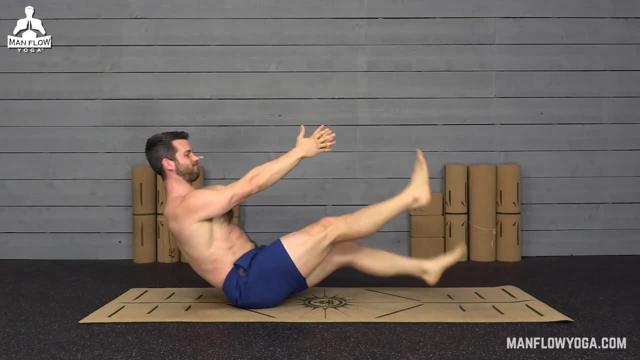 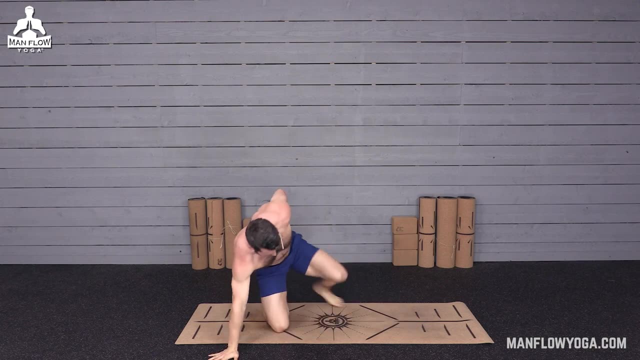 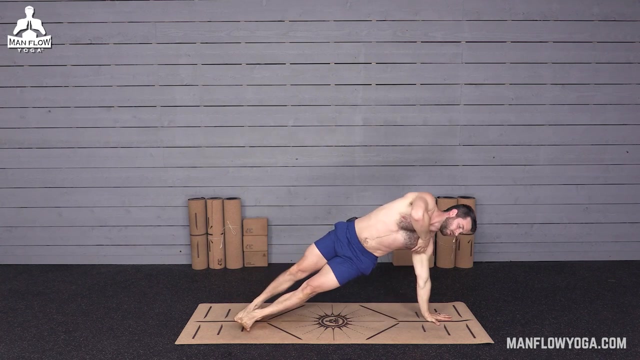 Five more seconds And then release. All right, good job. And here we're going to flip over onto your chest into a plank position and move into a side plank. So plant your left hand, stack your left shoulder on top of your left hand. 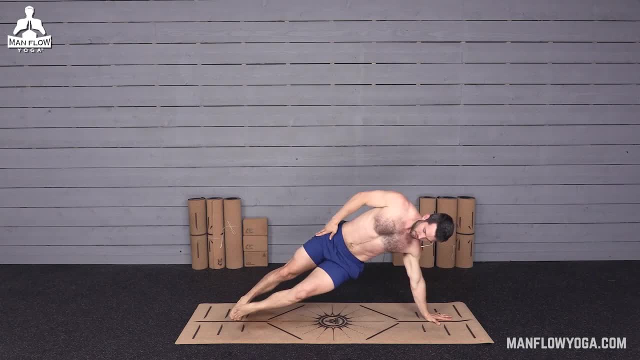 You can either start with your knees down. if you'd like, You can also stagger your feet or stack your feet. if you have the strength to do that. You're going to inhale to reach your arm up and then exhale. reach your hand under your body, kind of look under you. 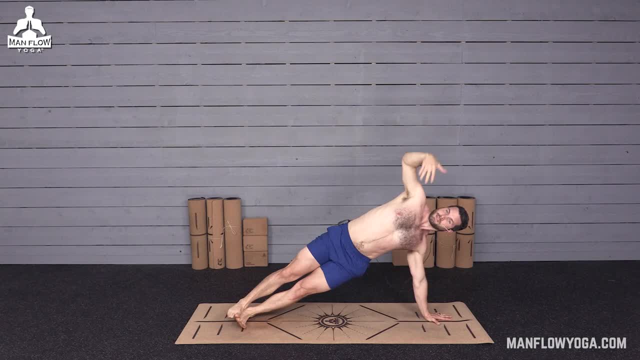 And then inhale, reach back up, Exhale, reach through. You can do five of these. Keep your hips driving up. This is really good for your shoulders, Really good warm up so that you're using your body properly, using your shoulders properly. 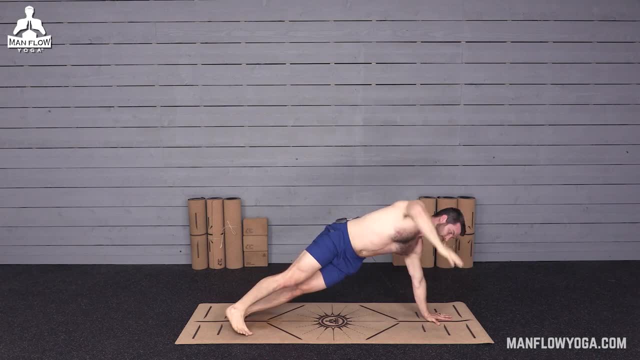 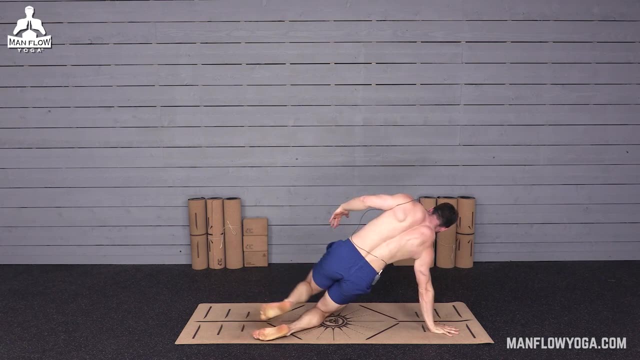 so you don't get pain in your shoulders. And then we'll switch sides. Point that right hand, roll to the right side, drive your hips up Again. lots of variations here. You can have the knees down and stacked, Stagger your stance or stack your feet. 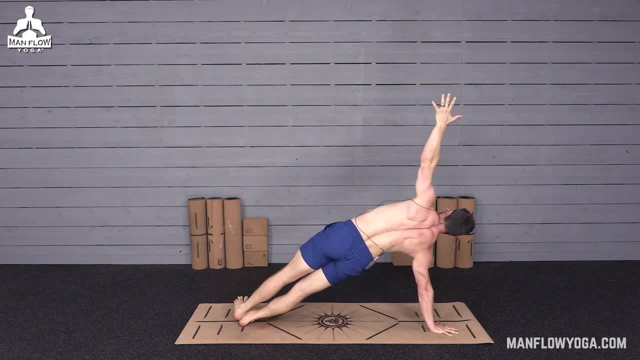 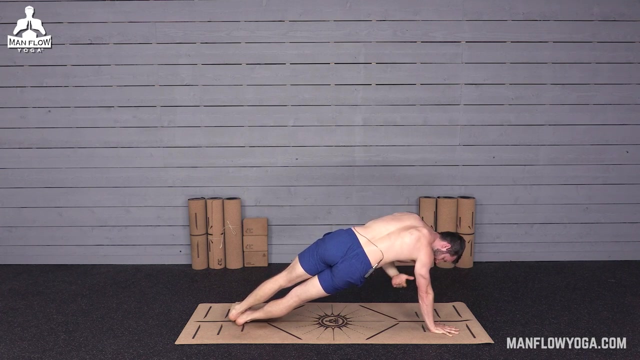 Reach your left arm up, Inhale As you exhale. reach your hand under your body, Inhale back up, Reach it through Back up And then five total of these And again. this is really good for your shoulders. 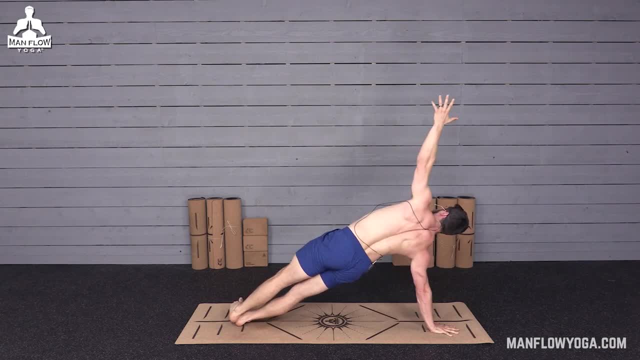 You want to make sure that you're doing these exercises with good technique and getting the right muscles involved. Otherwise, you could injure yourself, And that's a lot of what we do in these workouts. So you're going to notice that, If you can do these consistently, all right. 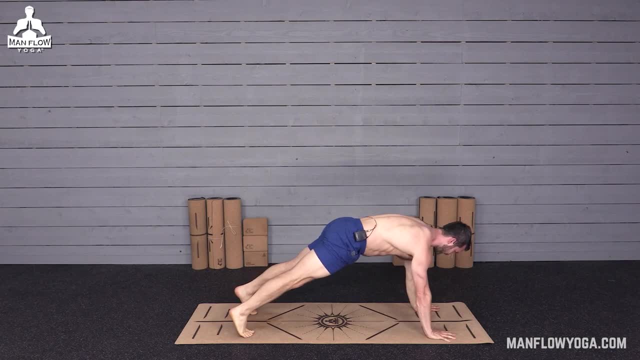 now we're going to plant, the hands coming into a plank, Hands under your shoulders, toes tucked, chest pulling slightly forward. breathe in and out of your nose. Lift your belly button up. Make sure your back isn't sagging here. Squeeze your feet and your hands toward one another. 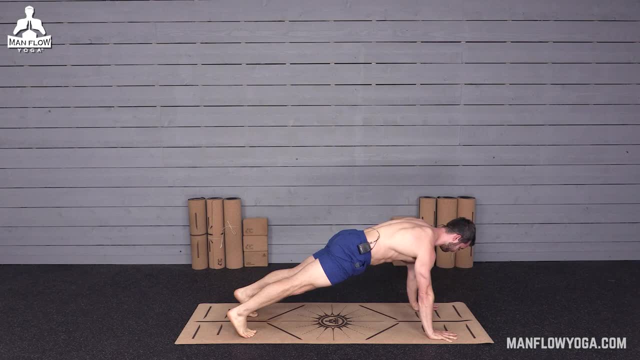 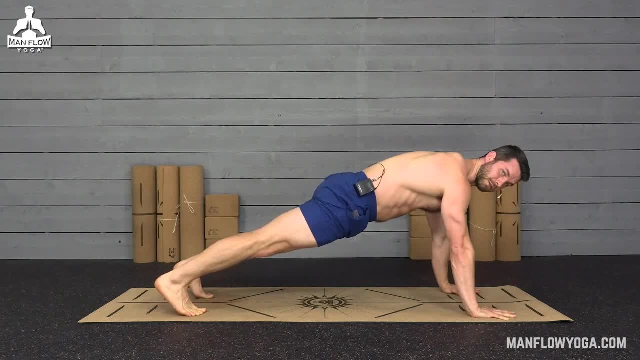 Breathe in and out of your nose. Breathe in and out of your nose Again. what we really want to do here is build muscle, So work on squeezing your muscles: squeezing your thighs, squeezing your abs, squeezing your arms and shoulders. 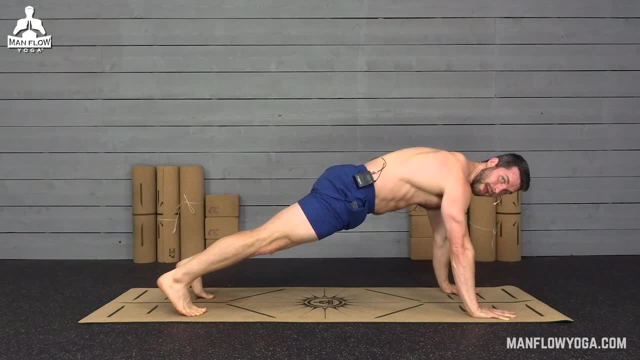 The more muscle that you can build, the more calories you burn at rest. So you can actually burn more calories when you're not doing anything. If you can build muscle, All right, go ahead and lower yourself down flat onto your chest From here. we're going to do some cobra rows. 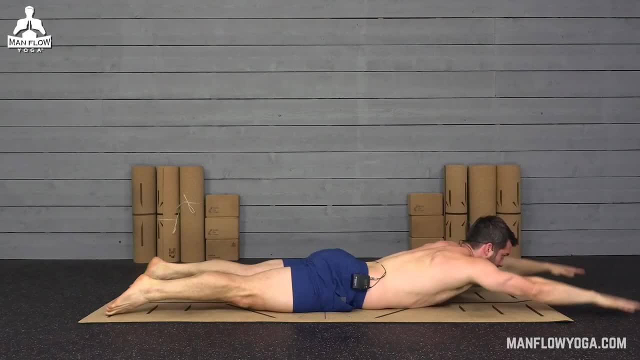 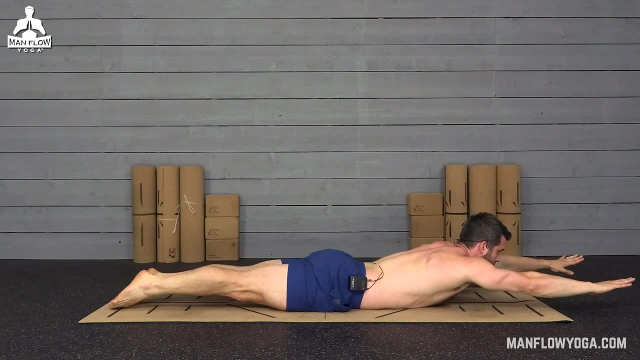 Extend your arms out in front of you, Lift your arms up off the ground, Extend your legs back, Point the toes, Squeeze your thighs together, Zipper up your legs and then inhale with your arms out. Exhale, Do a row. 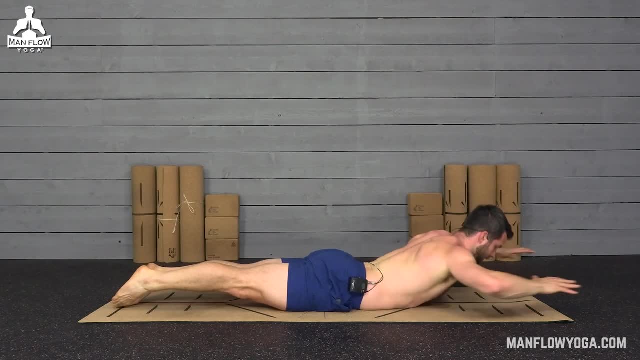 Squeeze your elbows back, Lift your chest back out, Inhale, Exhale Row 10 of these. Don't go too fast. The slower you go, the better. this is going to be, So if you want to slow it down, go for it. 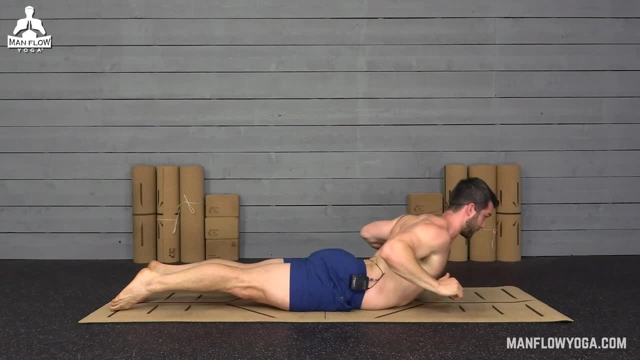 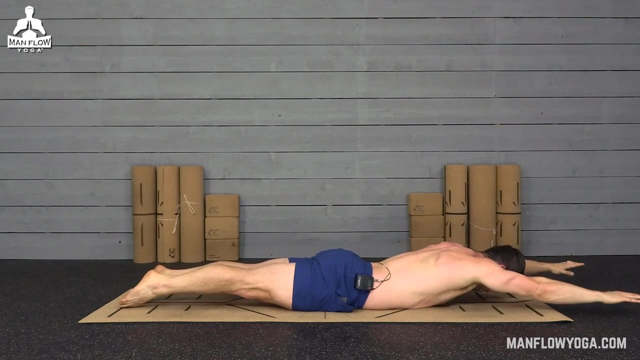 But I can understand why Moving fast is fun, So you're welcome to go fast. Make sure you're inhaling out and exhaling to pull in, Going up to 10 here. Make sure that you're squeezing your thighs and using your core to help your back. 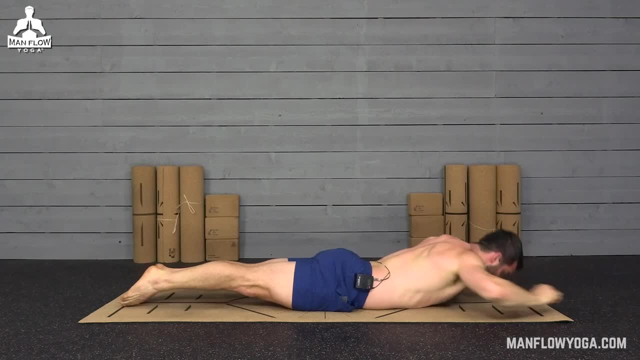 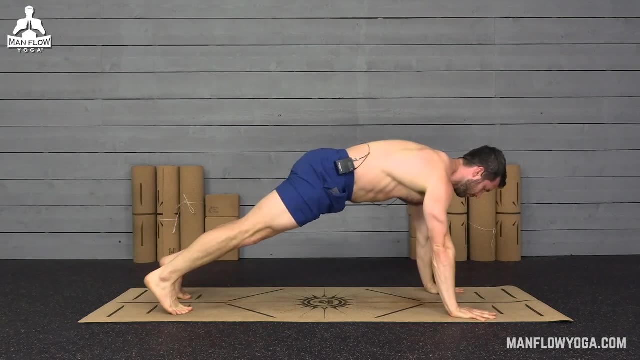 Shouldn't be all in the back. Last one, All right, and then plant your hands, Take it back into a plank, Hands under your shoulders. From here we're going to go knee to elbow, So Inhale. 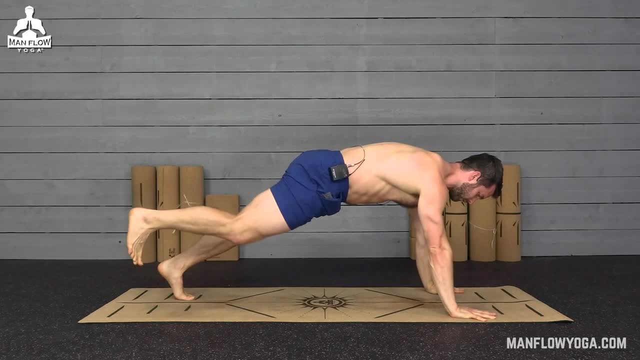 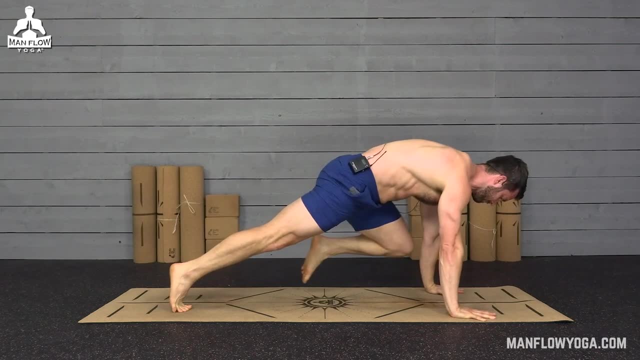 Inhale to get set. Lift the right leg up and then exhale Right knee, right elbow, Bring it back Inhale Left leg up and then knee to elbow, Switch sides and just keep this up at your own pace. 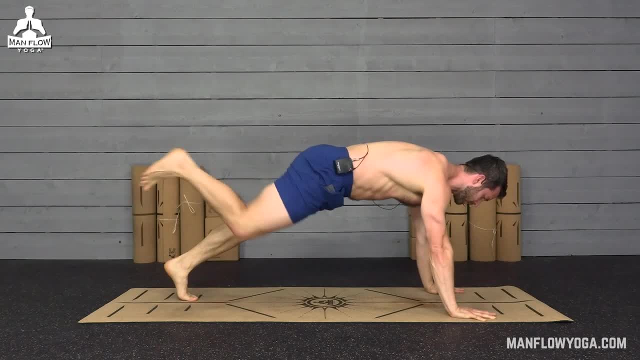 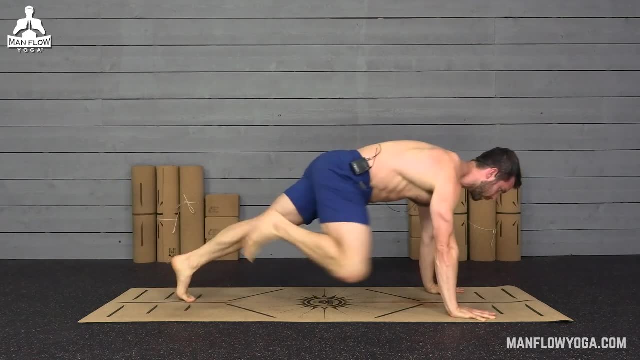 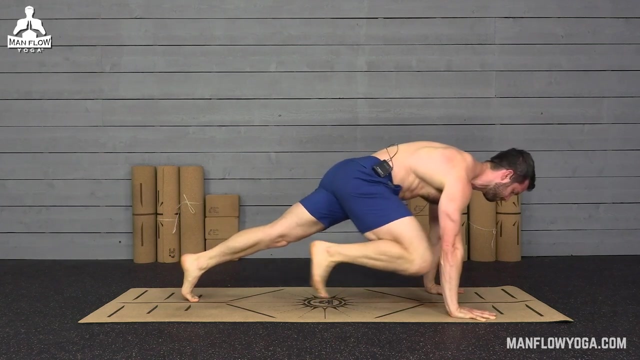 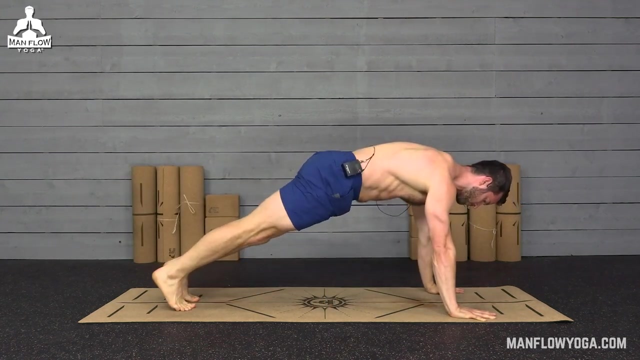 Exhaling to bring the leg in, Inhaling to bring it back. We're going to go three more to each side. So these really slow, controlled mountain climbers- Last one, All right, And then slowly release down on to your chest. 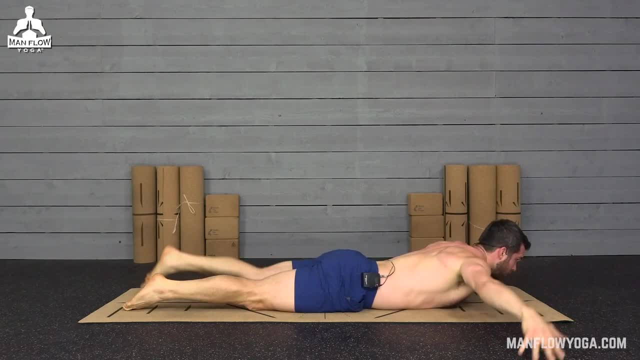 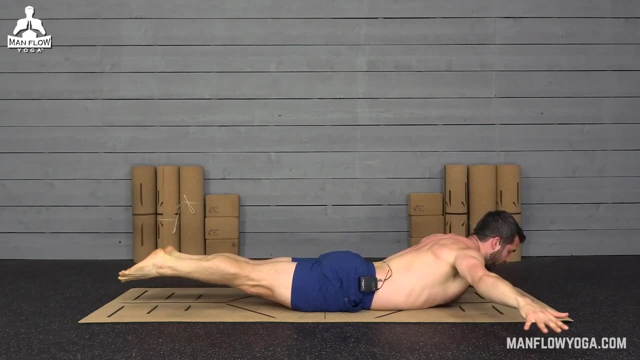 From here, you're going to bring your arms to the outsides, Reach your legs back again. Now I want you to lift your legs off the ground, squeeze your thighs and point your toes, And you're going to pump your arms up and down. 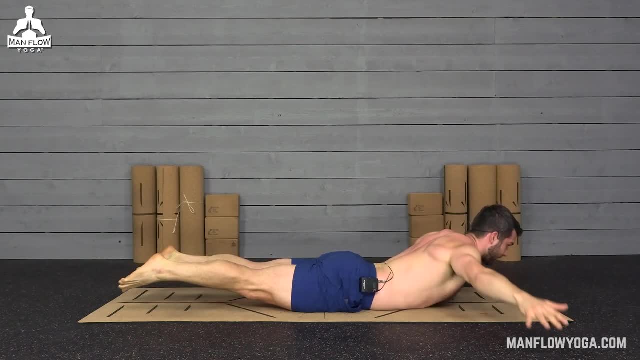 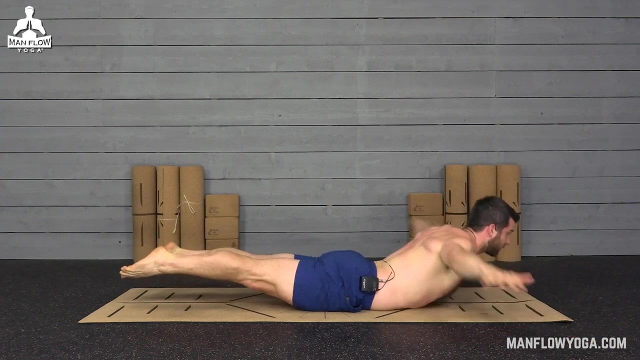 So squeeze the legs out, Squeeze up as high as you can, let them relax and then pump up again: exhaling to come up, inhaling to let it come down, going up to 10 here. Keep your legs pointed back. 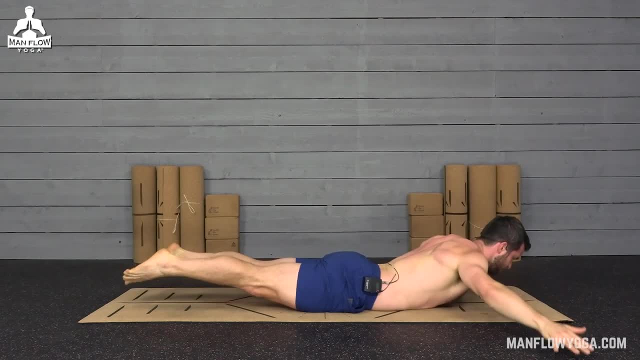 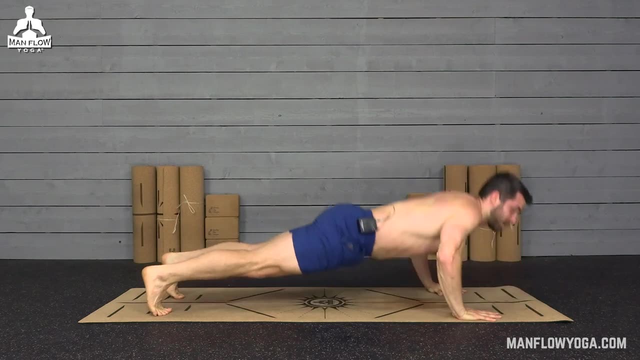 Keep your core working And then, on 10,, go ahead and plant your hands, Take it back into a plank position And from here we're going to go up into a down dog. Plant your toes, tuck your toes, I mean. 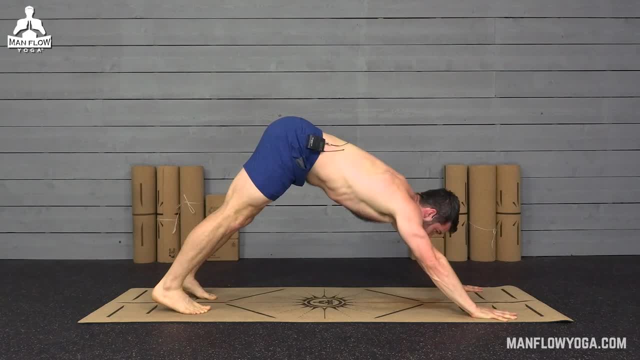 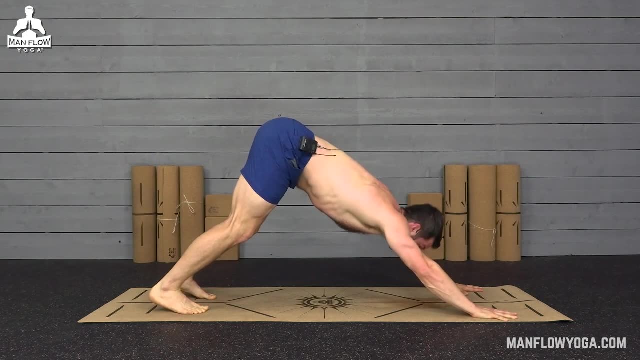 Press your butt up and back, squeeze your thighs. little stretch for the hamstrings. You can bend your knees if that feels uncomfortable for your back. Stick with me, guys. We got a couple more exercises to go. It's going to be a lot of fun. 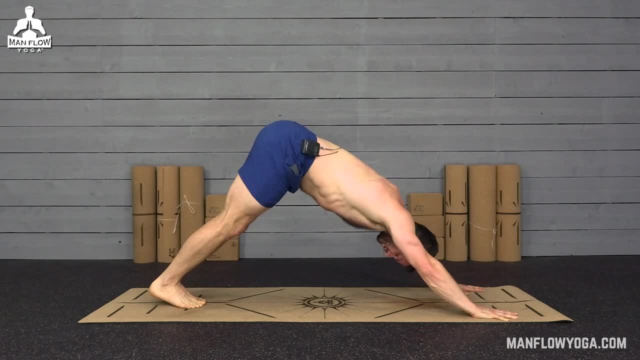 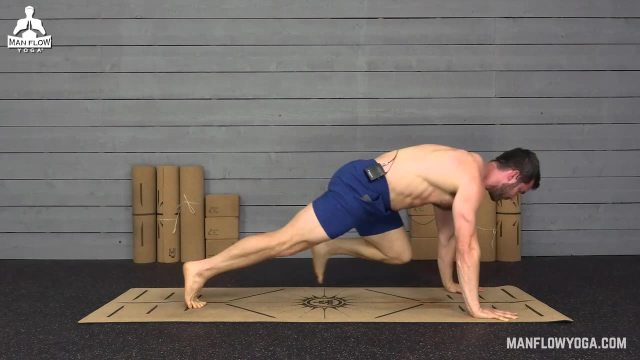 All right, bring your legs together, toes touching. Lift your left leg up, inhale And then, as you exhale, bring your left knee to your left elbow. Pull your body forward, Bring it back up to the down dog leg in the air. 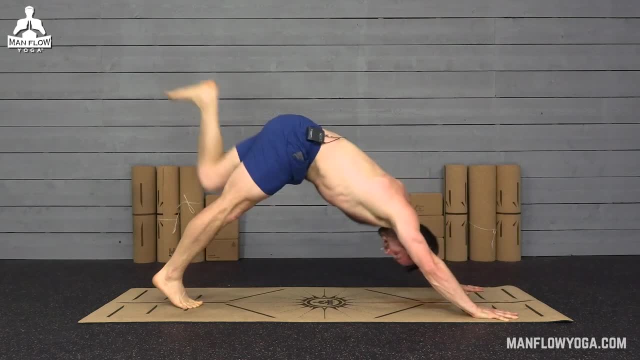 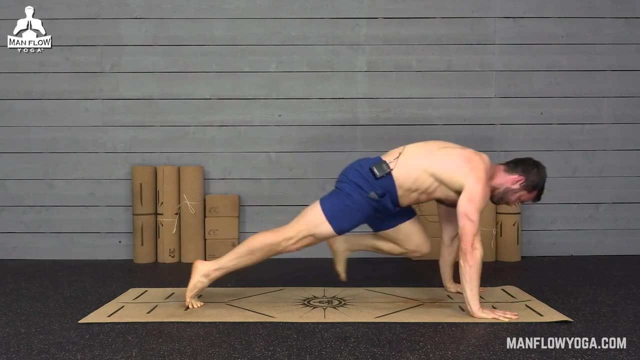 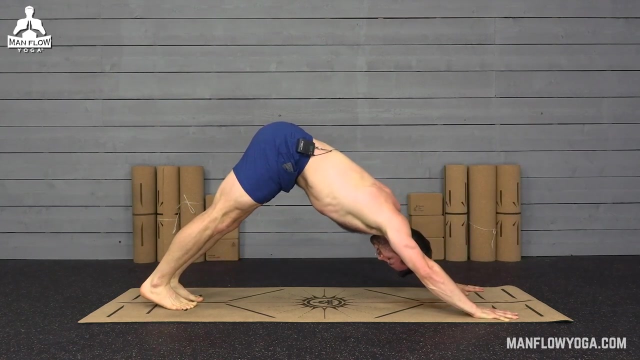 Again: left knee, left elbow, Back up, going to five of these, one more and then back to down. dog, Let your left foot come down, toes touching. We're going to go to the other side. five more, Other side. lift your right leg up, inhale. 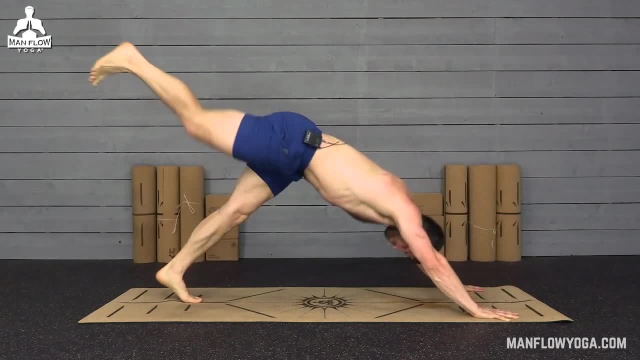 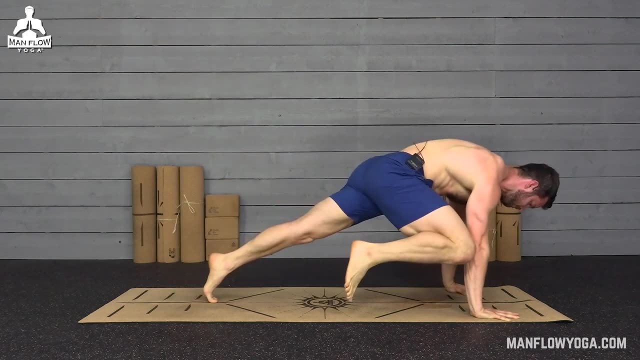 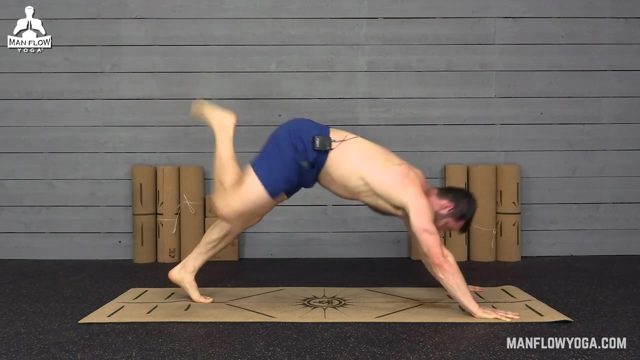 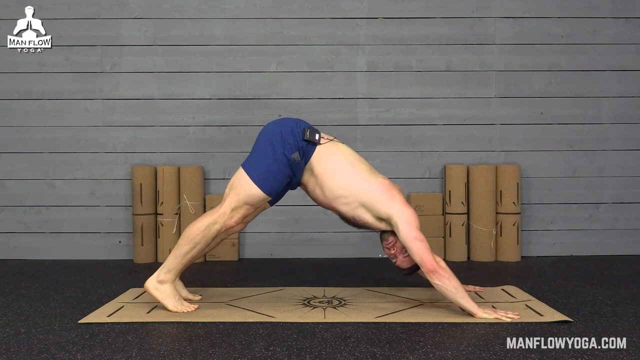 Exhale Right knee, right elbow, Inhale back up, going up to five, All right back to down. dog Guys stick with it. Got one more really fun exercise here. Remember you want to be consistent with these. 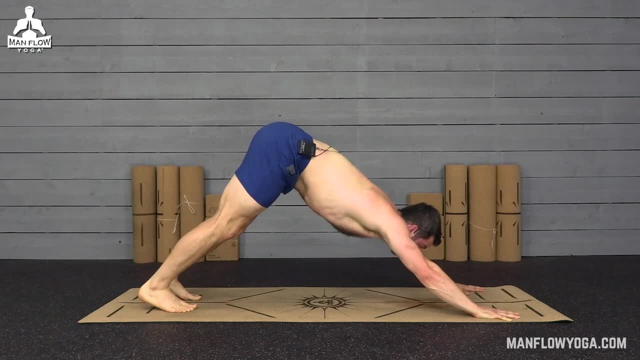 If you really want to lose weight, make sure you're doing these workouts three times per week. All right, Back to that plank Now. spread your feet as wide as you can on the mat. Bring your right arm out in front of you. 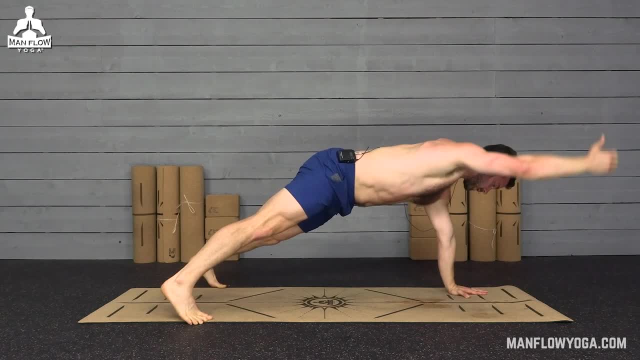 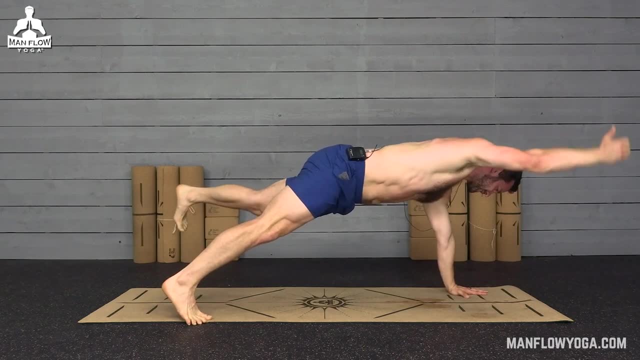 Turn your thumb to face up And you're going to pump your arm up 10 times: One, two, three, four. You can make it more challenging: Lift your left leg up to balance, Go up to 10.. And then switch. 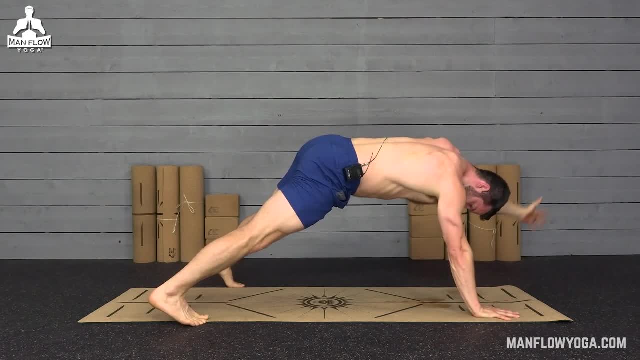 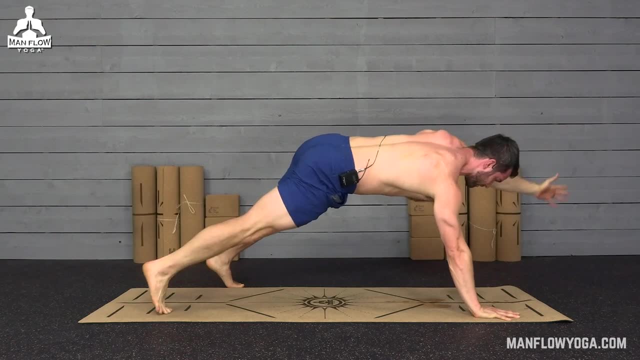 Plant your right hand. Bring your left arm out, Pump up to 10.. Left arm: squeezing up as high as you can, fast and strong, Maybe lifting that right leg to make this more challenging. And then plant that hand, All right. 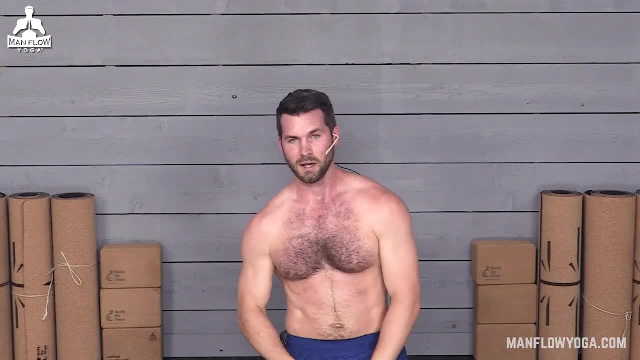 And release. All right guys, that's the workout. Hope you enjoyed. I've got another workout that's really good for building muscle. It's just 10 minutes long, full body. If you enjoyed this one, I think you're. 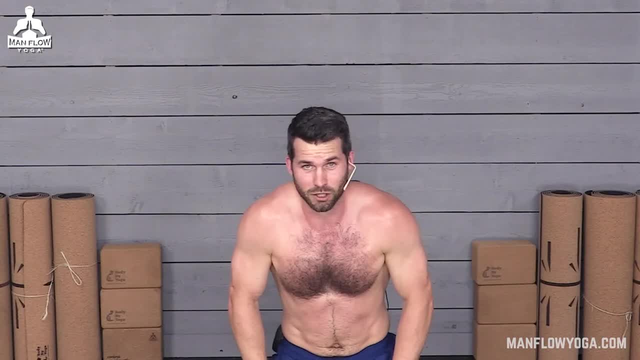 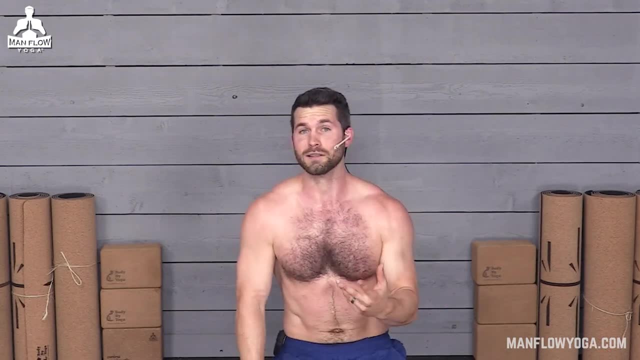 really going to enjoy that one. You can even stack these workouts. make it a little more challenging. Click over here to check out that workout. right now, We've got more workouts coming out every Tuesday at 9 AM. More workouts And this weight loss series are coming every week. 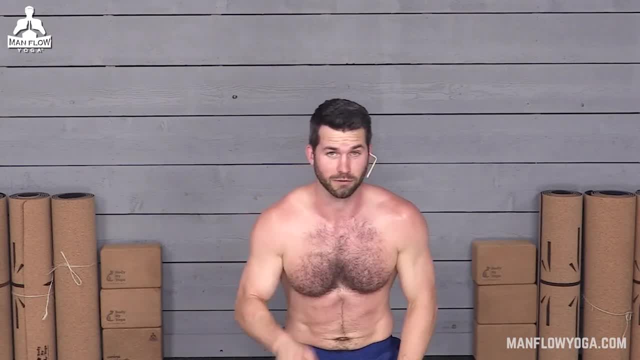 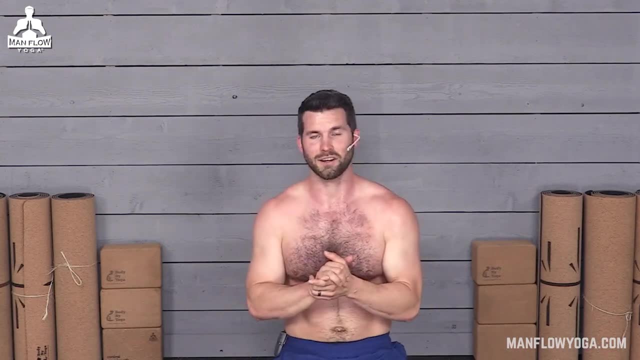 So for the next few weeks. so subscribe, Don't miss out on those Turn on notifications. If you like this video, hit the like button, Leave a comment if you have some feedback And I'll make sure to see you guys on another video soon. 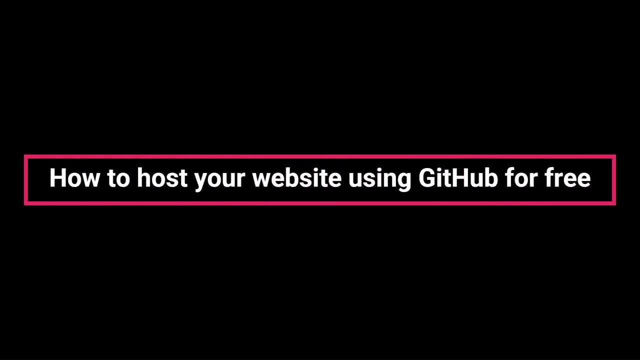 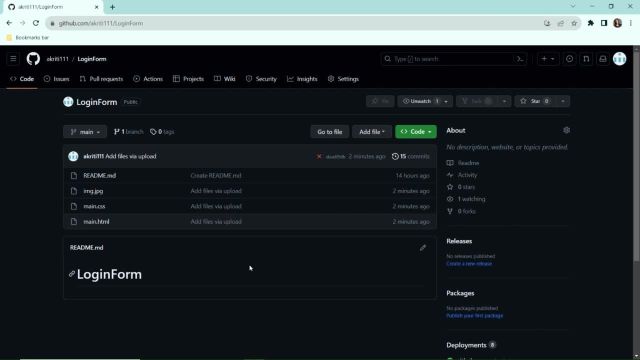 Hey guys, in this video I'll show you how to publish your front-end website using GitHub for free. So here we have a repository that has three files- mainhtml, maincss and an image- And if I scroll down a bit, you will see that this project is 65% CSS and 35% HTML. 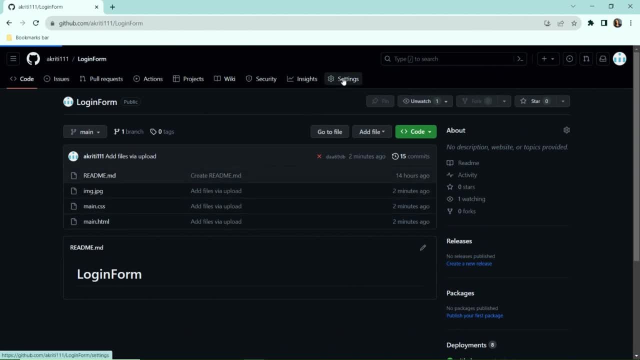 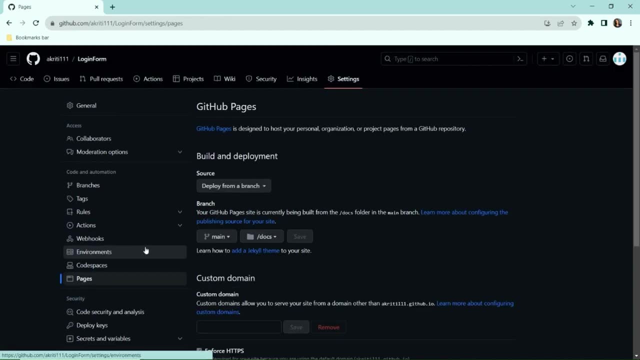 So to begin with, let's go to settings. Next click the pages options. under codes and automation section, Select the deploy from a branch option for source and select the branch you want the code from. in my case it is the main branch. 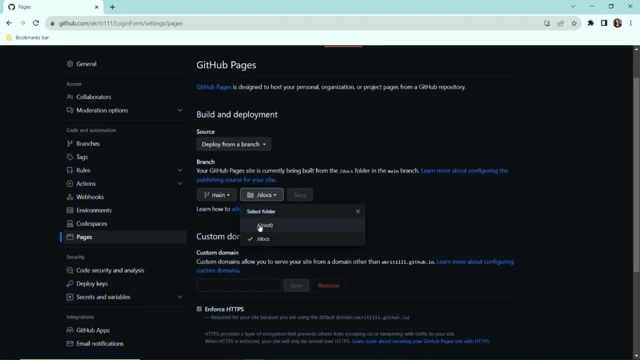 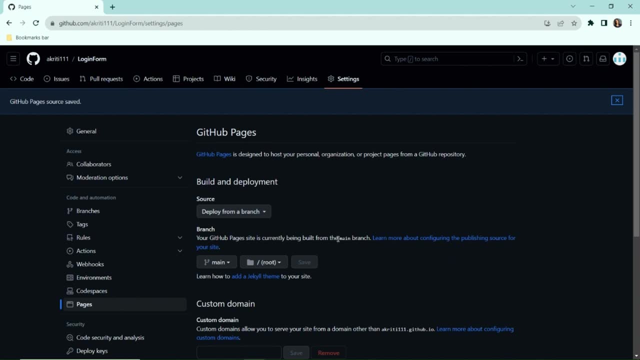 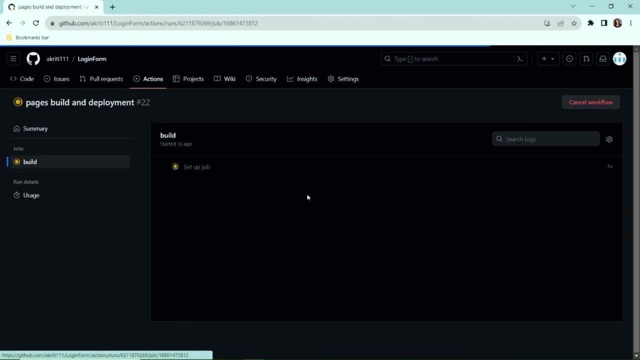 Then select the directory. it's root for me, because I did not keep my code inside any other directory. Then click save to save the GitHub pages source. Now go to code. you will see a small yellow circle. click on it and and then on details. 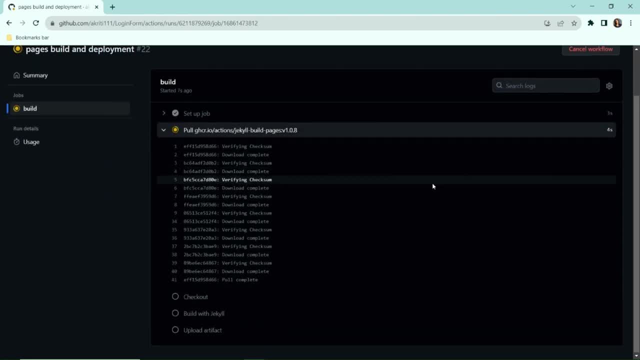 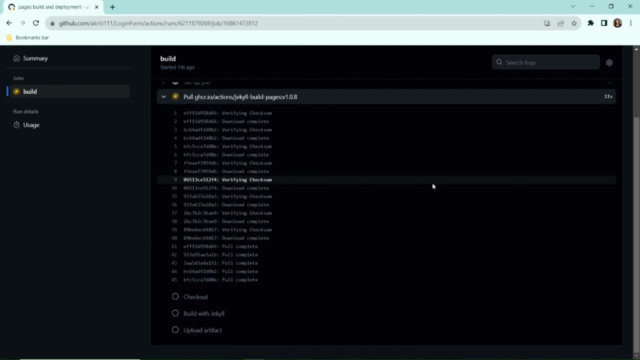 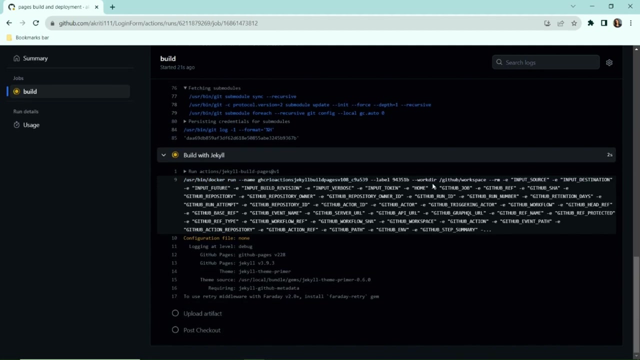 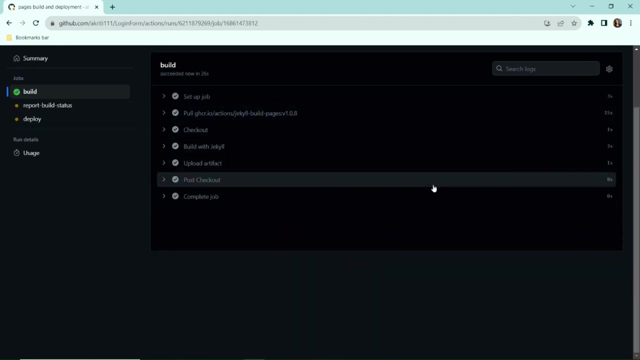 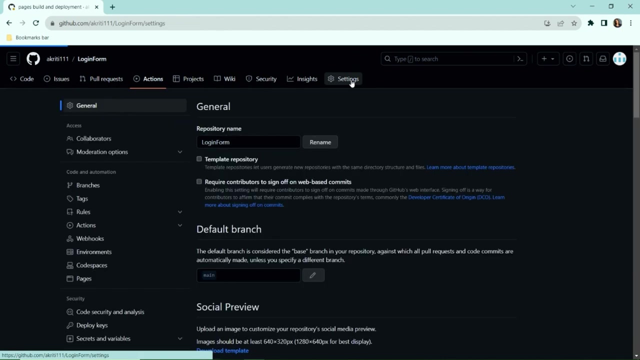 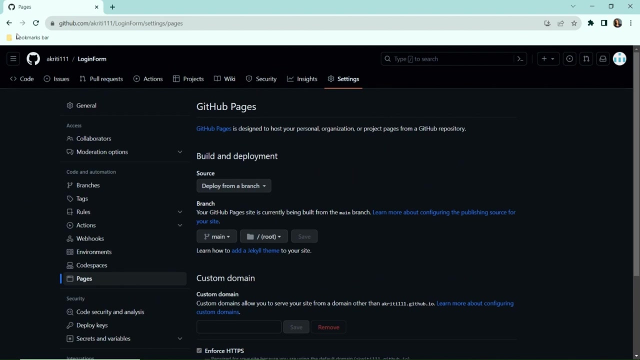 This shows the back-end processing of what's happening currently. Once all the steps are successfully complete, it's time to go back to settings And then pages. You will see your website link here in few seconds. Refresh the browser. Website is now live. we can click on this link or visit site option to open our website link.